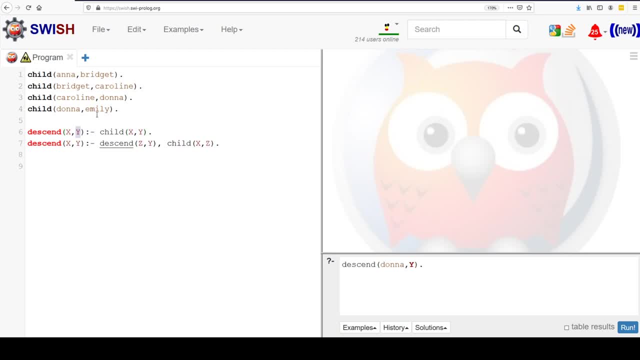 And this is going to be variable y, which we're going to be able to report back as a descendant. And so we're going to very quickly find that child of Donna is Emily And therefore we can descend. we have a descendant of Donna's is Emily. 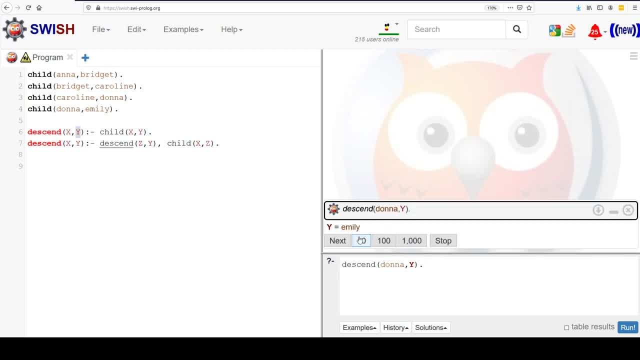 So let's run that real quick. Now we have a next here, Because there's still more predicates to search. right, We haven't searched the second descend predicate yet, So maybe there are more descendants of Donna. We don't know. 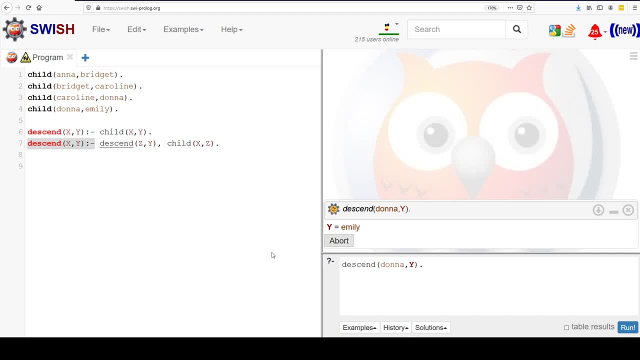 And so when we run this, this is where we get stuck in our infinite loop. So the problem here, as you'll see reported pretty quickly- is that we have a stack limit exceeded. This is basically an infinite loop, And so what happens is we dive in to this descend predicate. 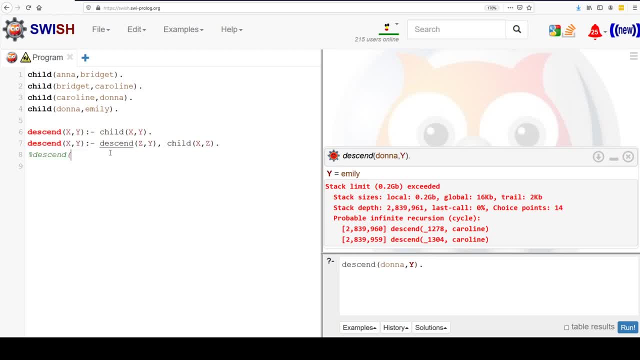 And so we're checking: descend If descend, and child x- or I guess x- is Donna. We've already unified that. And then z. So this z will ultimately unify with this z, This y will ultimately unify with this y, But right now they're all variables. 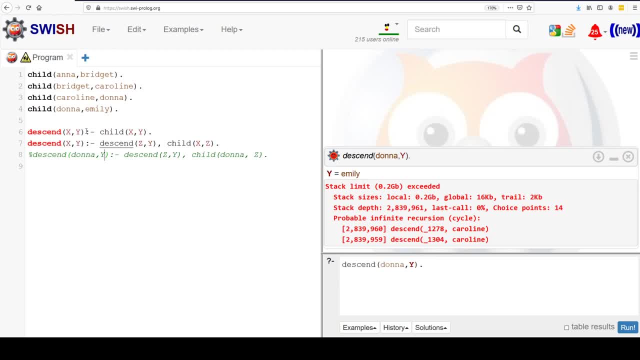 So basically we're saying who are the middle pieces here If we're going to search further down the tree, what other descendants could Donna have? So, the way this is ordered, the first thing that Prolog is going to have to evaluate is this descend. 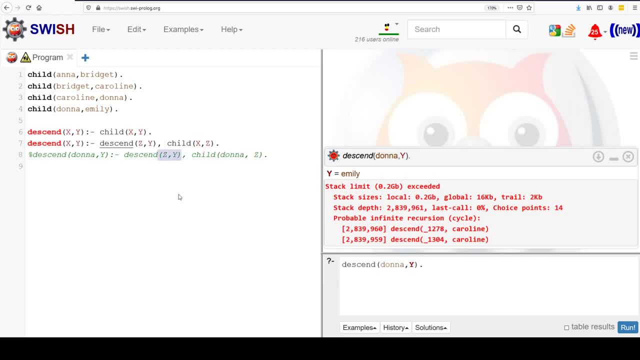 So we're trying to find a descendant of anyone. So any z, any y, What are my possible descendants? So we're going to try all the different combinations of children. None of them are going to yield a true result when we bring them back up and check up here. 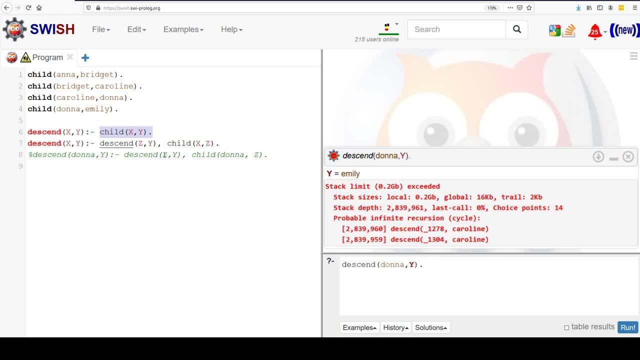 Because there are no other descendants of Donna. So we're going to see if there are various combinations of people that are further down the list of children here. If there's various other pairs of children that like, for example, if Emily had a child that we could find and match and work our way back up. 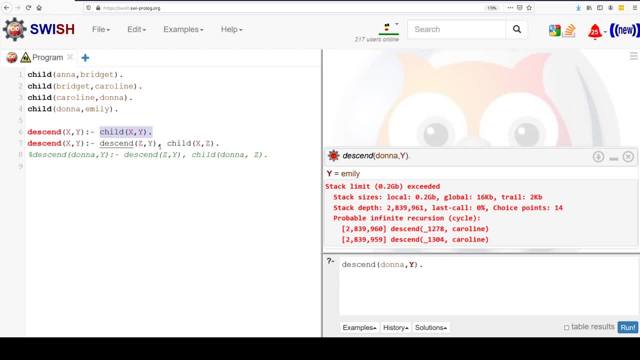 And so we're going to try all the possible combinations And none of them are going to work. But because descend is first, that means that we're actually going to have a potentially. We're going to infinitely call descend before, Even if we run out of all the child combinations, we still could potentially have descend combinations. 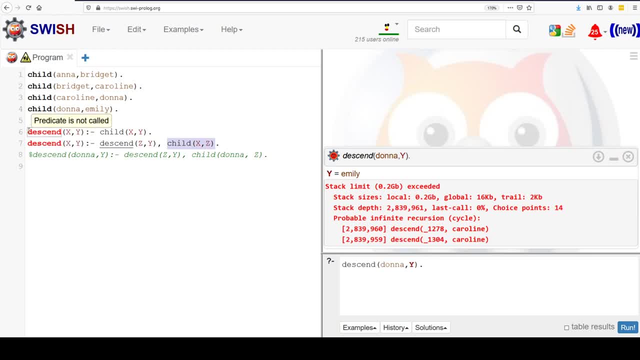 Because when we try a descend combination, this is going to eventually run out of options and we're going to get falses here, But here we're going to recursively descend. So, rather than actually walking through all the options and all the details and all the depth here, I think the most important takeaway is this: 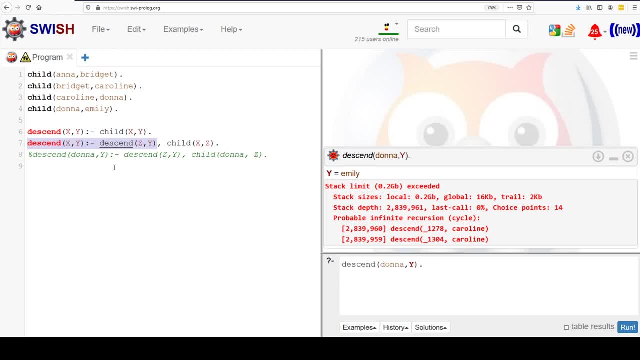 You should always put the non-recursive predicate before the recursive predicate or the recursive rule. So the reason for this, the principle, is that we want Prologue to evaluate the non-recursive goal first, So that if it runs out of options for this, if we do not have any possible children that would satisfy this, then we can really quickly stop searching. 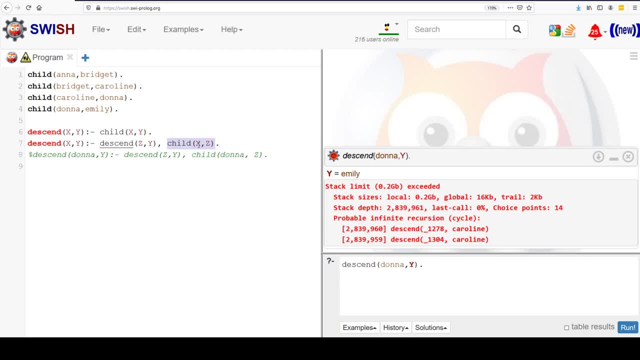 So if we're searching all the child options first here, Then as soon as we run out of child options to search, there are no more potential calls to descend Because, well, there's no more possible options here. If descend is first, then Prologue is going to try all the possible options of descend. 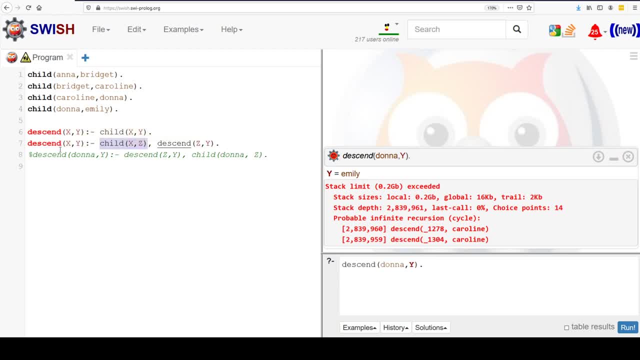 And since it's recursively calling itself first, there's no flag to it to stop recursively calling itself. If it runs into child first, it stops. This is like short-circuiting in Java. If it runs into child first, it stops. This is like short-circuiting in Java. 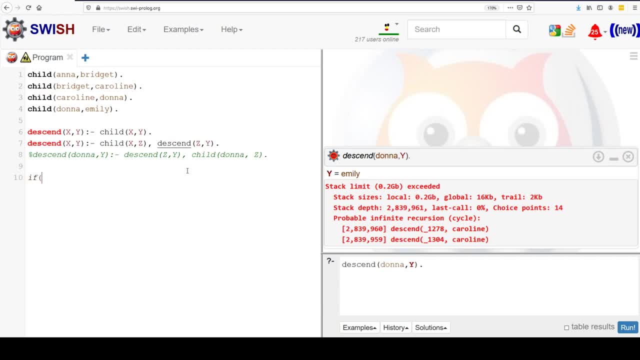 If you have an if statement. let's say, if x is greater than 3 and x is less than 17.. Well, you may not actually know this, but it's true. In Java, if the value of x were negative, 5.. 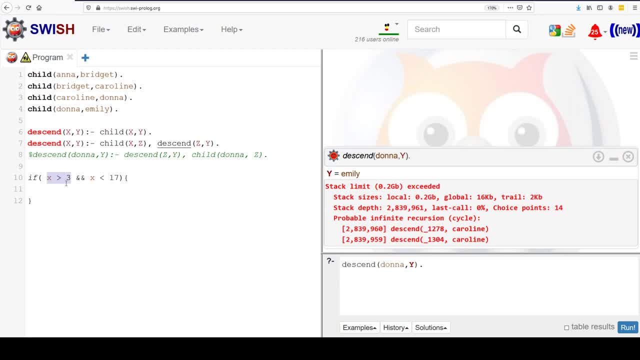 Well, we have an AND condition here. And x is not greater than 3. And x is not greater than 3.. So in Java the question, the check for x less than 17, is never going to happen. It's the same idea in Prologue. 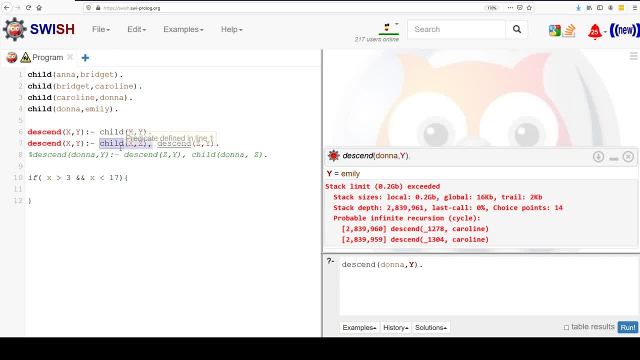 It's short-circuiting. If we run out of child predicates and there's no possible child predicate that could make this descend true, Then we're going to stop And we're not going to actually evaluate descend. If it's the other way, then we're going to evaluate descend first. 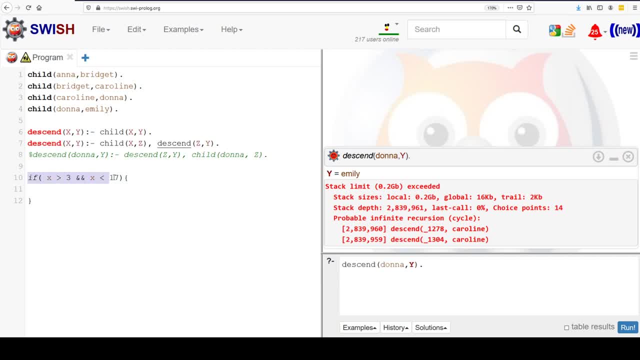 So, for example, in this example- I guess this is kind of where the example breaks down a little bit- But if we had an x value that was 100.. Both of these are going to have to be checked- 100 is greater than 3, so then we have to make the second check. 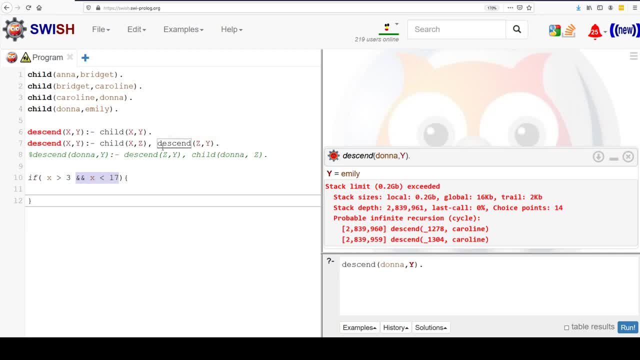 And so both happen. As it turns out in Prologue, though, it's the recursive call that's the only dangerous one. So it's almost as if this call- You know, we want this call to be the dangerous one- that could recursively loop and check things. 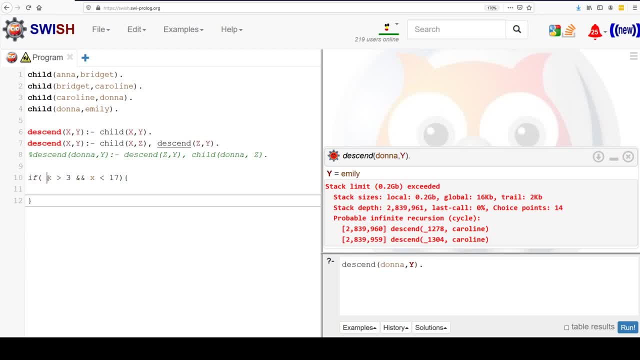 And this call to be the easy one, So that if we can easily remove something from consideration, we never do the more dangerous recursive call. Hopefully that makes some sense. This comparison doesn't work exactly because these are both the same level of risk or the same type of call in Java. 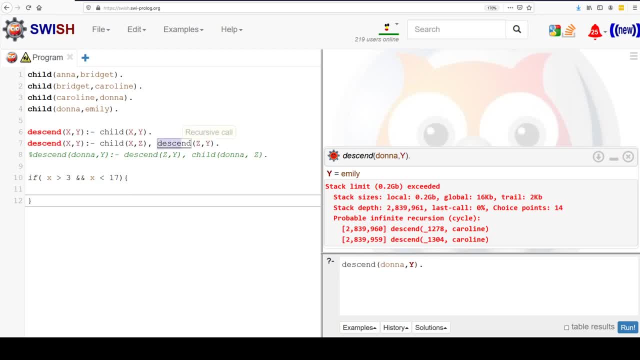 But in general in Prologue you want to avoid putting recursive calls first. You generally want to put recursive calls at the end so that you can short-circuit your way out of them. So the difference between this example is that we have one dangerous call and one safe call. 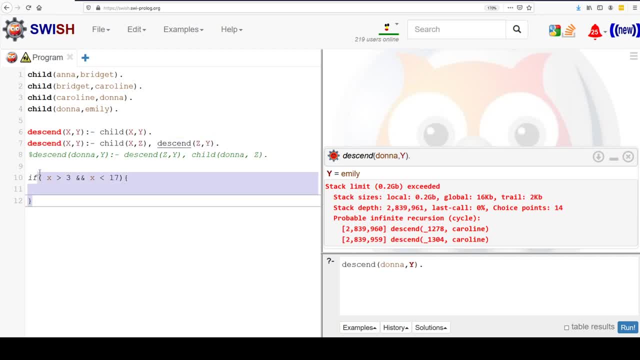 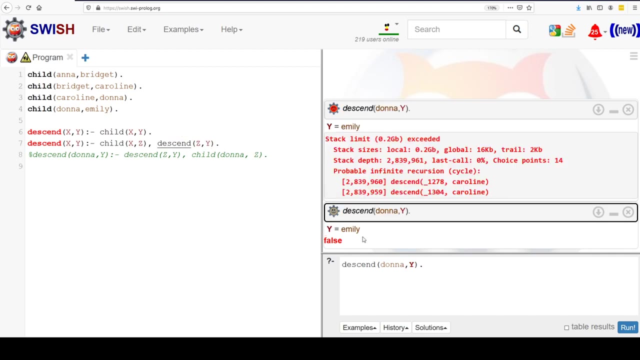 You want the dangerous call at the end so you can short-circuit your way out of it more often. So that's probably more important than knowing the details about how the infinite descend tree works. Note that, just to prove that this works, if I run with descend, at the end we find our first, Emily here. 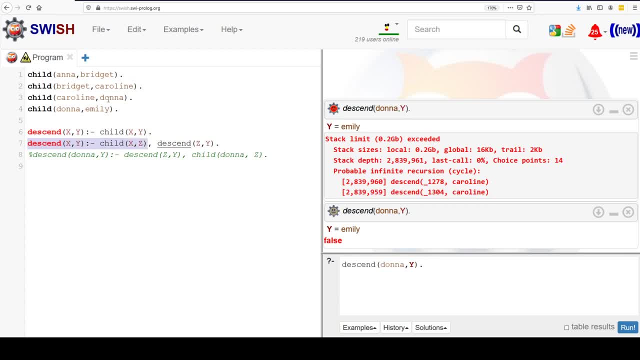 We then check our descend predicate. We try to find all the potential children that could work and therefore check if they are descendants. So we're going to do some of this, But once we run out of all the child options- child pairs- then this will evaluate to be false. 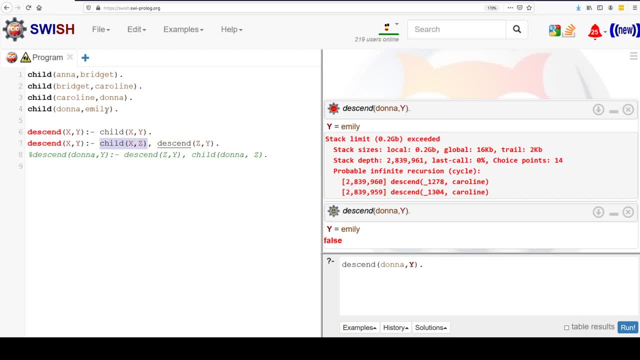 Because no child pairs were found that worked, and we've evaluated all the different child pairs, So therefore, this gets short-circuited out And we no longer actually check the recursive call, which leads us away from getting into an infinite loop.